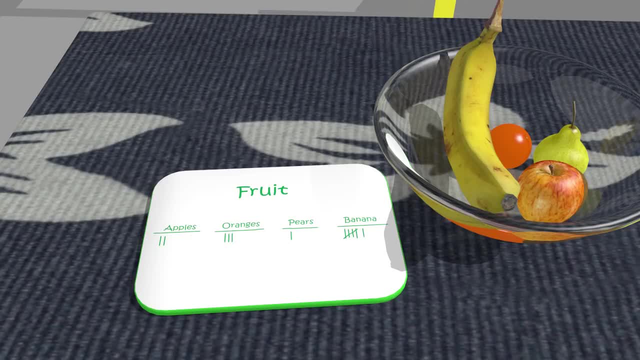 Here you can see that I have tally marks to show how many of my friends liked which fruit most. You might know already, but a tally mark is a useful way to represent data. Each time a friend told me they liked a certain fruit, I would put a tally mark under that. 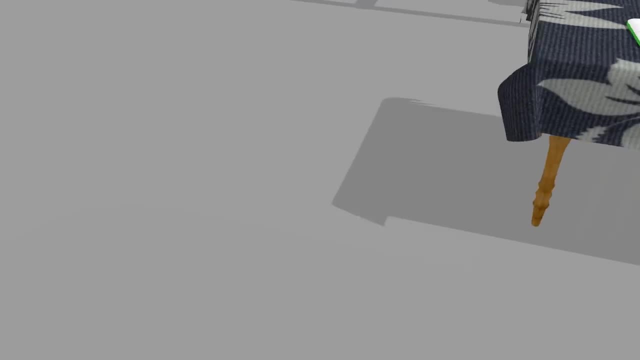 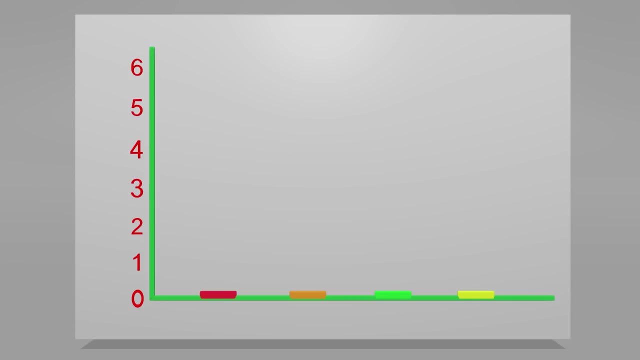 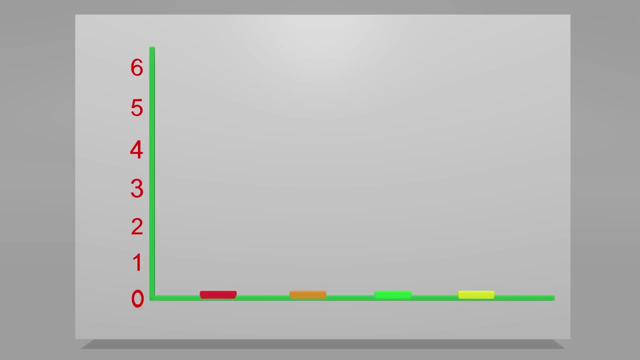 Here is a bar graph. Here is a bar graph. But the first thing we need to do with any graph is what We need: a title. Since the information we collected was on favorite fruits, let's call it Favorite Fruit. With this graph, I want to put the names of the fruit on the 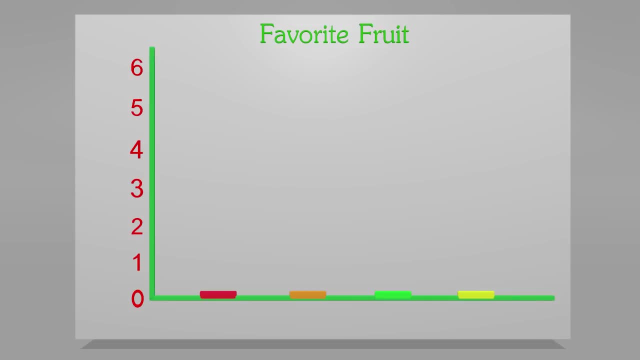 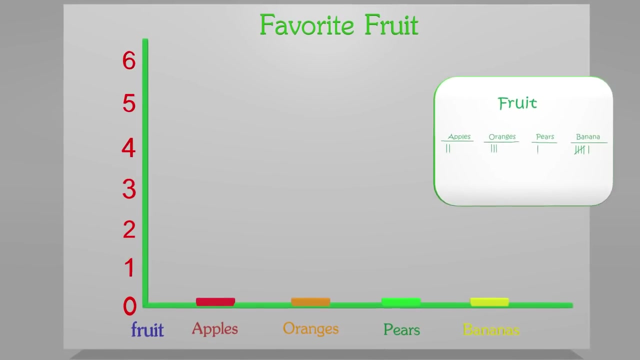 bottom and the numbers on the left side going up. We can see here on the bottom we have the names of the fruits. We should label what these are. This is obviously going to be a be labeled fruit. since they're fruit On the side, we need to measure how many. 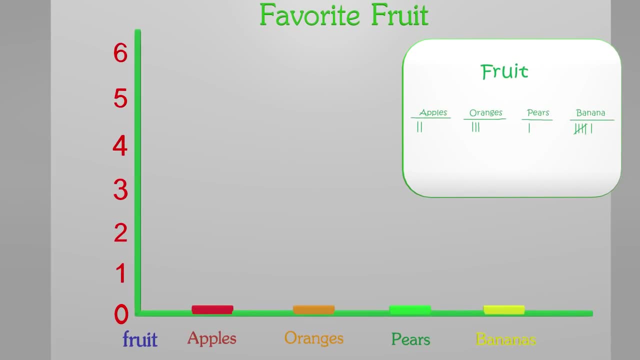 people liked these different types of fruit. We only need to go up to 6, since our information or tally marks only go up to 6.. So the numbers going from 1 to 6 represent the amount of people. We can now fill out the graph according to. 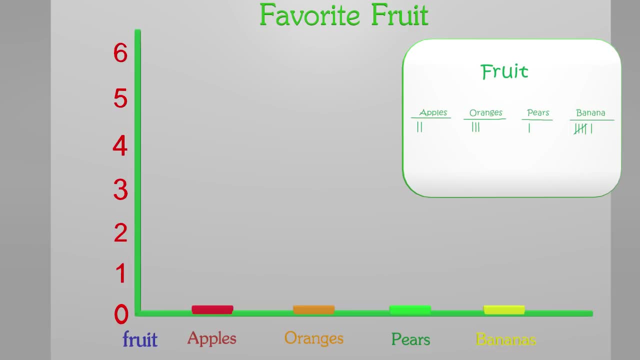 our data. First in our data are the apples. We can see from the tally marks that two of my friends liked apples. So here on the graph we will have this bar at the bottom. go up two spots to show that two people liked apples. Ok, next we have oranges. How many people? 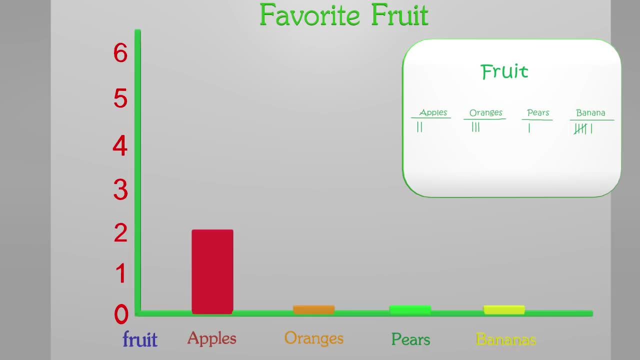 liked oranges. Good job, Three people liked oranges, So we move the bar up to where the three is. Now, how many people liked pears? We had just one that liked pears, so the bar goes up just one. The last one is bananas. 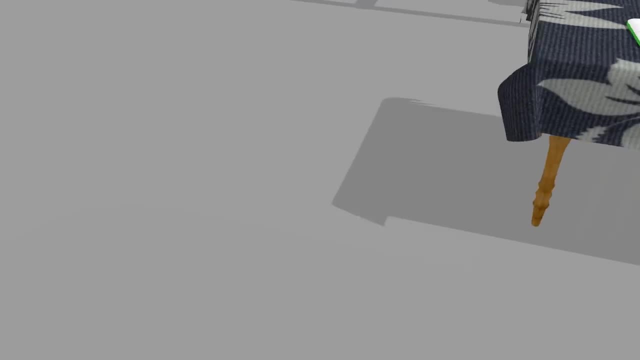 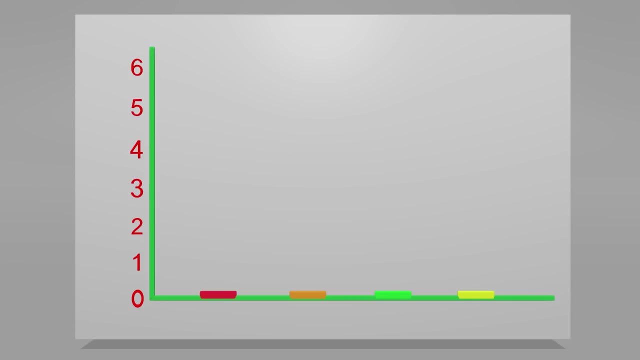 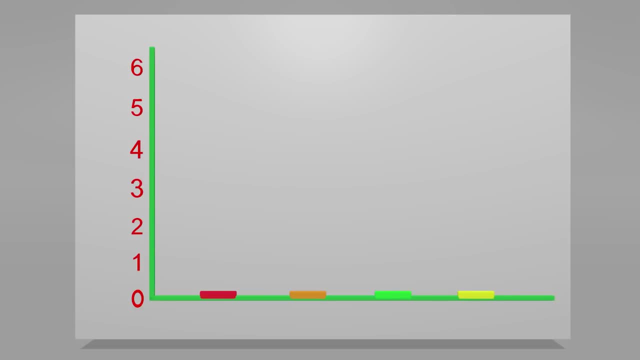 tied to the bottom of the chart, so all the values needed to fall into the number head of the curve work in a reading. Here is our graph, but the first thing we need to do with any graph is what We need a title. Since the information we collected was on Favorite Fruits, let s call it Favorite. 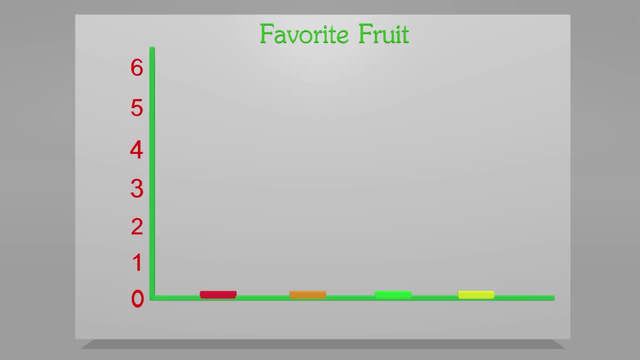 Fruit. With this graph I want to put the names of the fruit on the bottom and the numbers on the left side going up. We can see here on the bottom we have the names of the fruits. We should label what these are. This is obviously going. 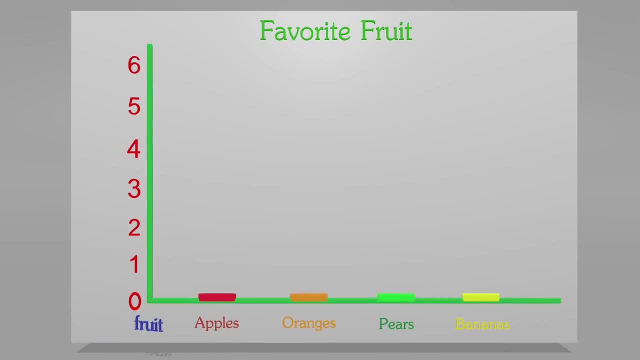 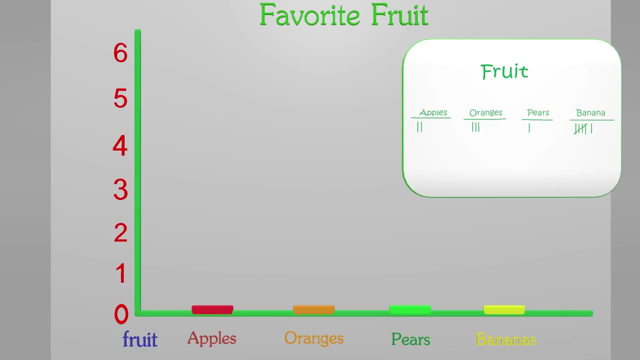 be labeled fruit, since they're fruit On the side. we need to measure how many people liked these different types of fruit. We only need to go up to 6, since our information or tally marks only go up to 6.. So the numbers going from 1 to 6 represent the amount of 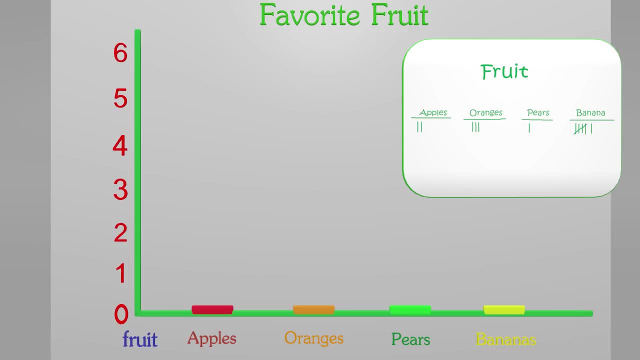 people. We can now fill out the graph according to our data. First in our data are the apples. We can see from the tally marks that two of my friends liked apples, So here on the graph we will have this bar at the bottom: go up. 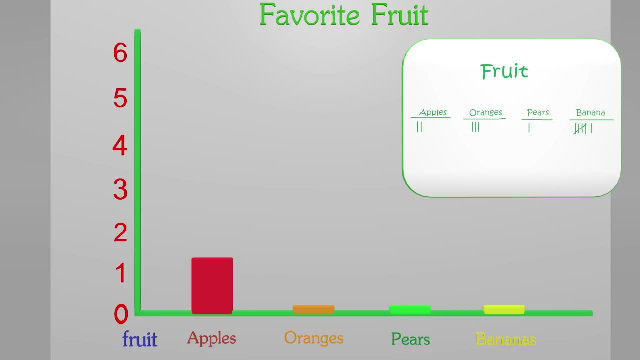 two spots to show that two people liked apples. Ok, next we have oranges. How many people liked oranges? Good job, Three people liked oranges, So we move the bar up to where the three is Now. how many people liked pears?